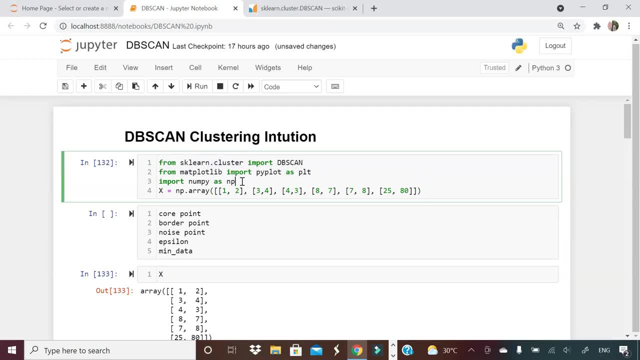 I'm taking matplotlib and then pyplot, I'm importing numpy as np and I'm creating this simple data here, guys, if you can see 1, 2, 3, 4, 4, 3,, 8, 7, some data points, right. 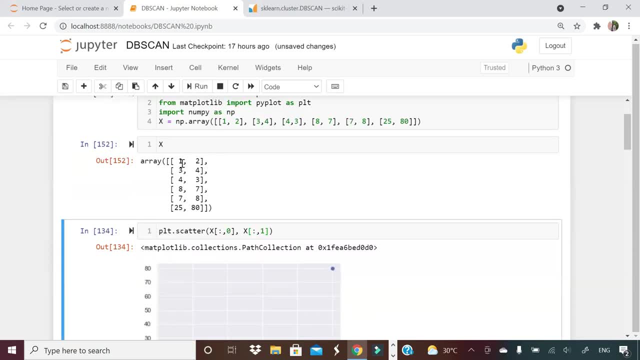 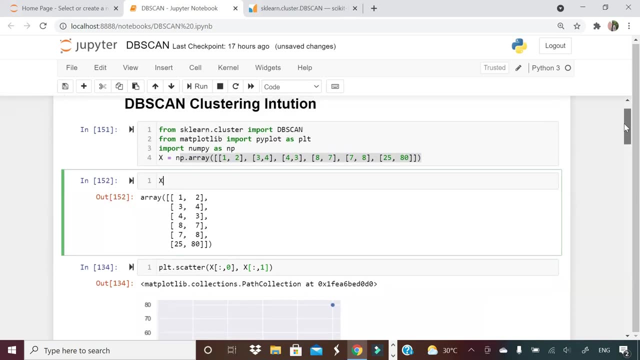 So let me run this first. Let me run this. So this is how my X looks like. Okay, so this is my X, which I have created. Now, by looking at this X guys, what do you feel? If I give it to a clustering algorithms, then how many clusters will be formed? 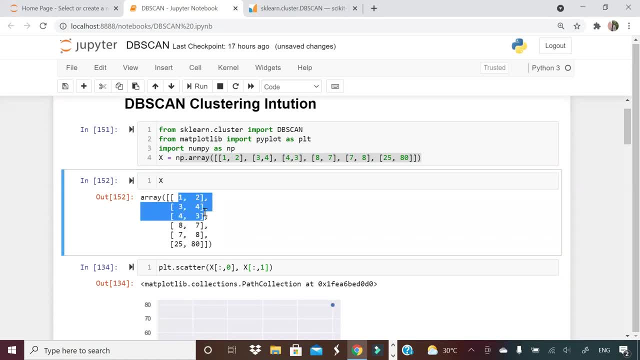 So let's see here guys 1, 2, 3, 4 and 4, 3, these three points are close to each other. Okay, Hence I'm assuming there will be one cluster for these guys, then 8, 7 and 7, 8,. 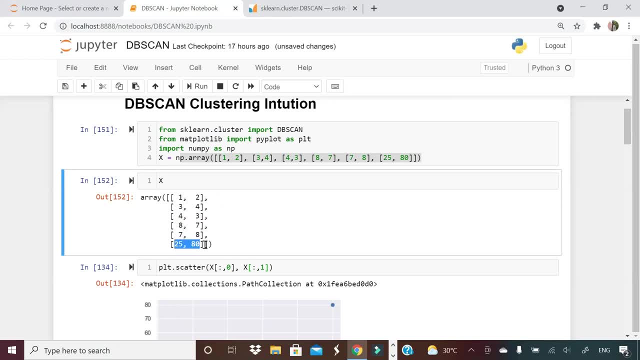 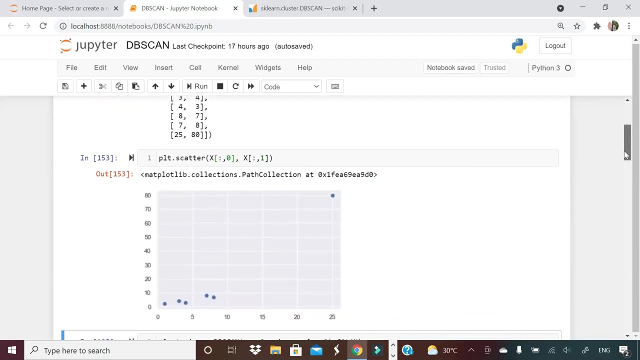 maybe one cluster for this And one data point I have knowingly put far. The reason for that is: I want to see if this goes as the noise. Okay, So now, if I plot this X, right, if I plot this X, which I'm doing here, you can see that. 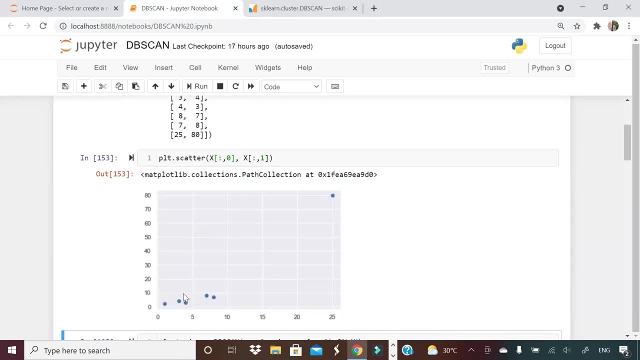 There is a three points together here, right, Two points together here, And one point is very far. This is nothing but the last point. Okay. So how DB skin clustering works, guys, is it will try to find out the density of points. Okay, So wherever more density is. 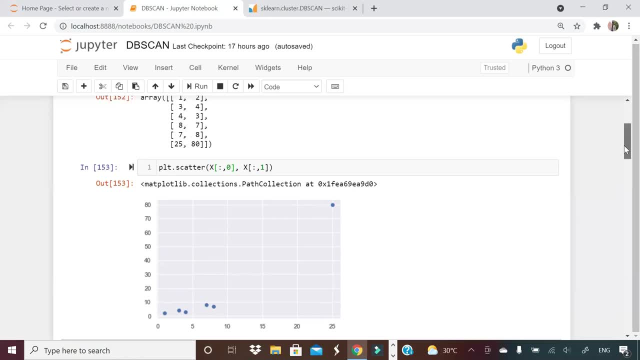 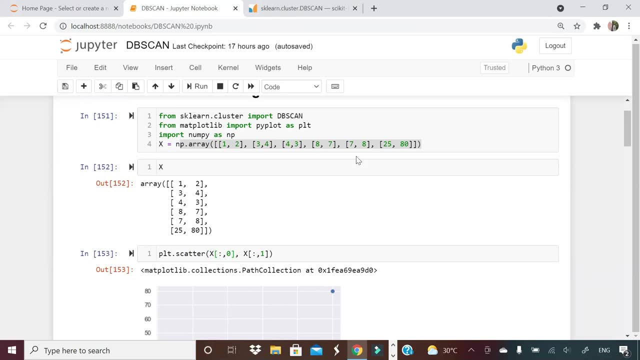 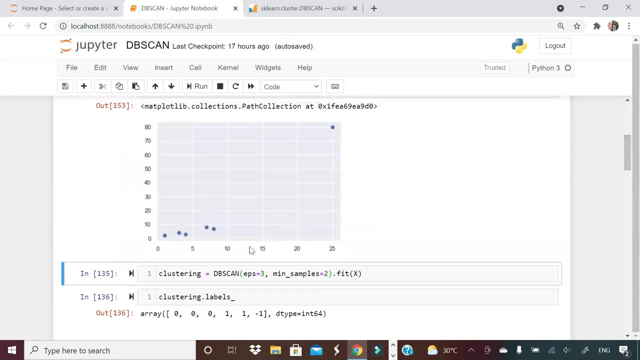 there it will say that it is one cluster. based on what? based on those five things that I wrote here: core point, border point, noise point, epsilon and minimum sample. Now let me call a simple DB scan clustering On top of this data. Okay, So how we do that? I just go here and say clustering is equal. 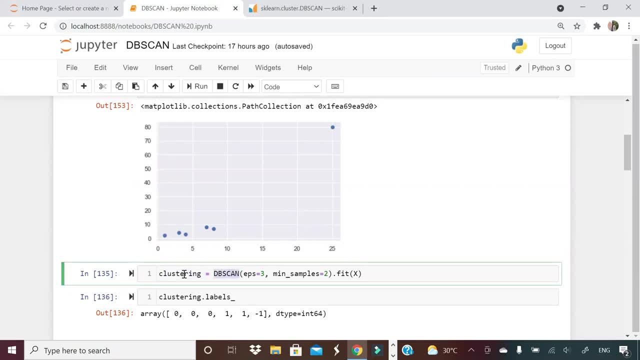 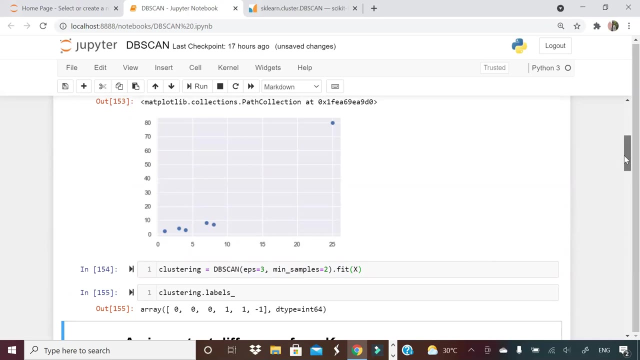 to DB scan, and DB scan will necessarily take two parameters, Guys. One is epsilon and other is minimum number of samples. And then I call it fit on which data? on X. Okay, Once I run this, guys, you will see that there are how many clusters formed here. Clustering dot. 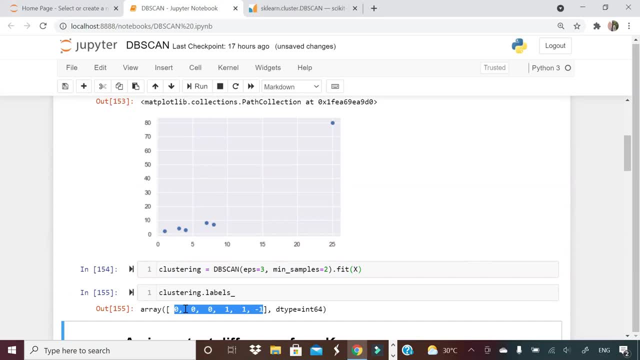 levels. If I say you can see zero, one and minus one, three different values, Okay, So what? what the Python is saying us is: your first three data points fall in cluster zero, Your next two data points fall in cluster one and your last data point is a noise. So 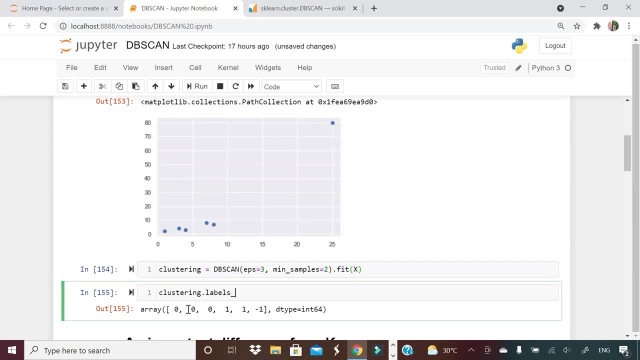 always remember these guys. whenever you run DB scan, you will see some minus one levels. Okay, The meaning of minus one is: it is a noise. Noise means something which is far, which is neither a border point nor a core point. Okay, Now see here two important parameters. 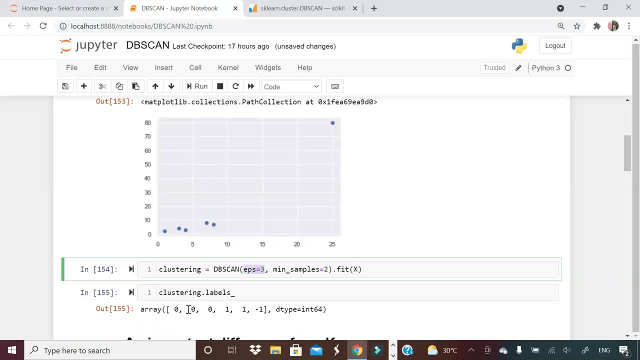 Guys. One is epsilon. So what is epsilon? epsilon is nothing but distance of closeness, For example, what you call as close based on Euclidean distance or Manhattan distance. The meaning of this is: if I reduce this right, what will happen is the, the, uh, the. 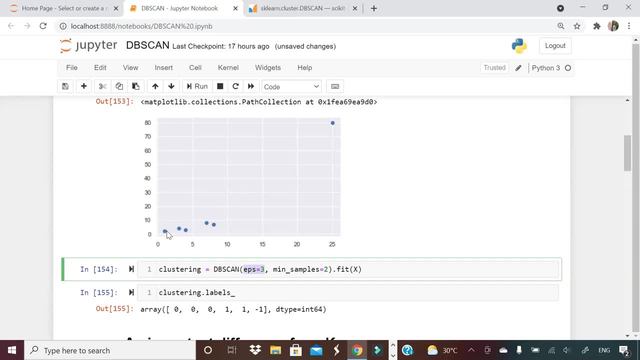 idea of clustering will be different, Which means, if you see here, these two points will be having some distance between them. Okay, Which is less than three, And hence there is two considered as a one cluster. If I make it from three to nine, right, What will happen? 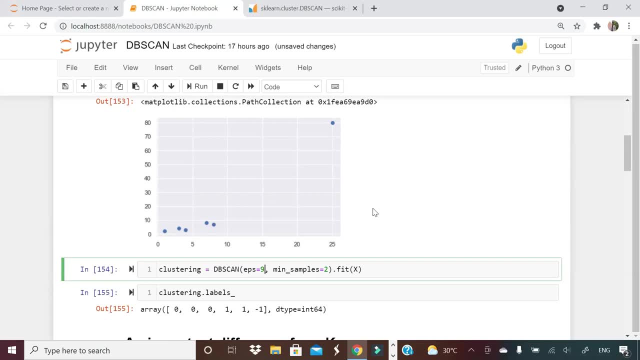 My number of clusters will increase or decrease. My number of clusters will decrease. The reason being: I am saying something which is nine, you know, nine units away. That is also close for me. Consider that as close for me. So let's run this and see how many clusters now. 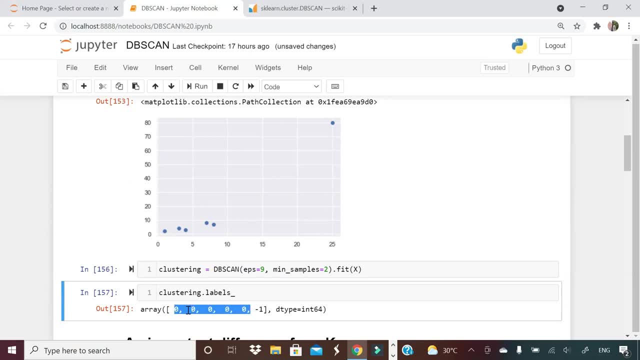 As you can see, there is only one cluster: zero. Okay, What I have done? I have increased this Epsilon, which means I'm saying: consider the far points also as something close. That is how Epsilon works, guys. Here minimum number of samples is two. What happens if I make? 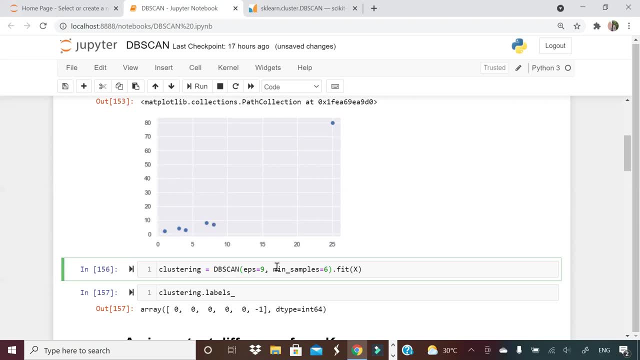 minimum number of samples at six. What happens, Let's see. So what will happen is all the data points are considered as noise. What is the reason, guys? The reason is, in total, we have six data points, only, right, And what I'm saying is that the data points are considered as noise. So what is the reason? 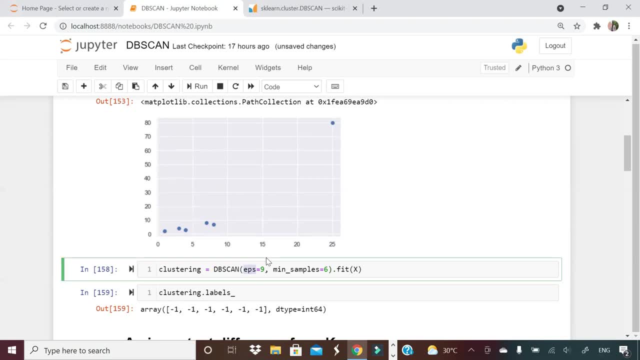 what I'm saying here. I'm saying: take Epsilon nine and your definition of core point is only if you have six samples. So there is a possibility that this point is more than nine units away from all these points or core point. Okay, And I'm saying, if there is not, 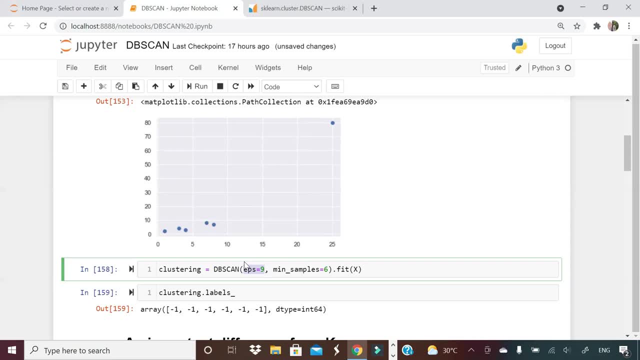 six samples inside your one cluster don't define any cluster. So if don't define any cluster means all these things will be called as noise, Hence minus one minus one minus one. Okay, Now, all these things I have taken from directly SKlearn page guys. I will just show. 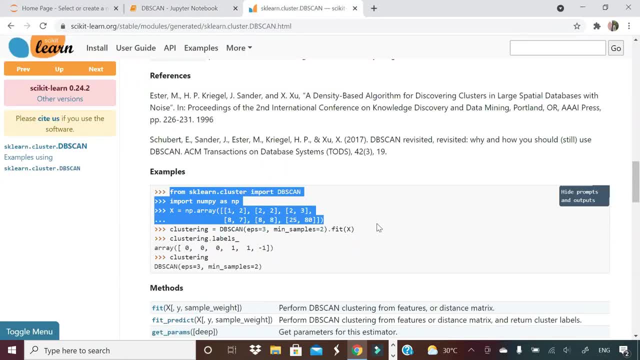 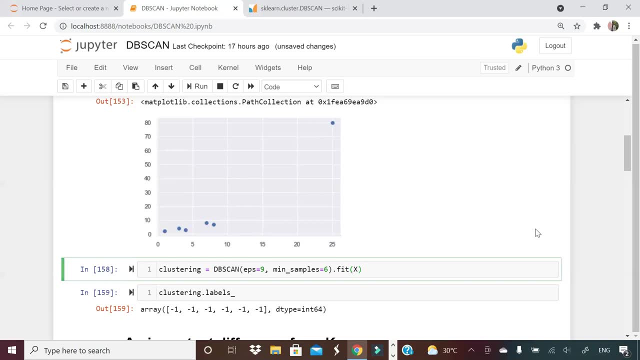 you here, If you can see here everything. all the example definition is from SKlearn page, only till now. Now I want to show you one important thing which is different in DB scan clustering interview question, also as compared to K-means clustering. Okay Now. 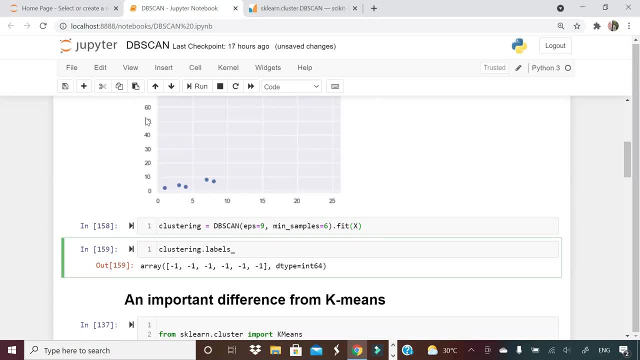 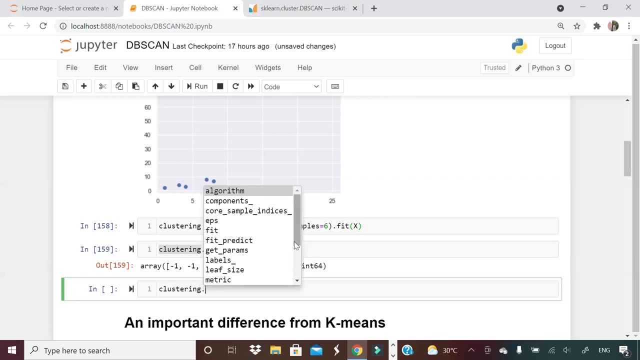 guys, if you see here I have fit a clustering model here right? So I should be able to predict on the new data, right? So clustering is nothing but my model. So clustering dot- if I press a tab I expect a predict function here. But if you see, there is no predict function. 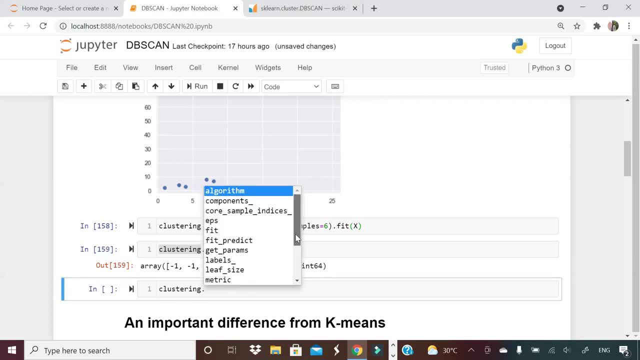 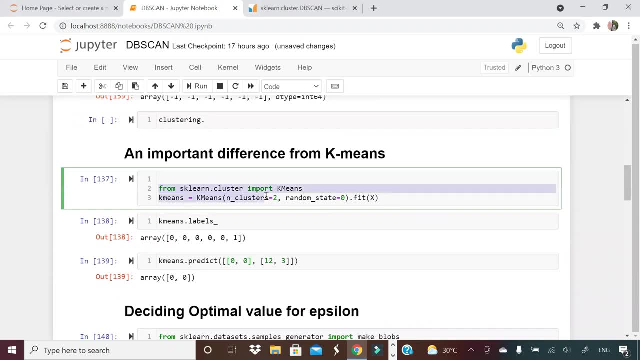 guys, I will tell you the reason why it is not there. There is no predict function, Okay, But if you fit a K-means model here, see here I'm importing K-means. K-means is equal to give me two clusters fit on the same data. Let me run this: K-means levels, How many clusters? 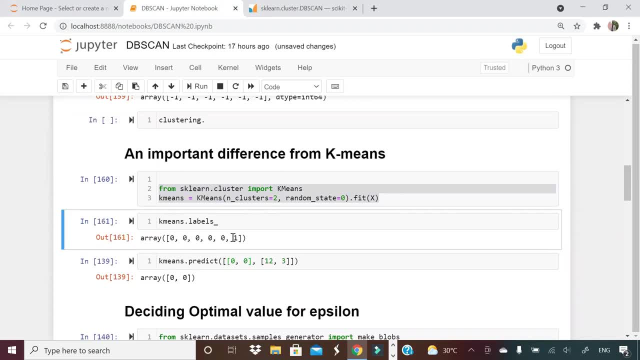 K-means is giving one cluster five data points, other cluster only one data point. And then I can very well run a predict guys, K-means dot predict and some input data. It says that your both these input data falls in a cluster number zero. 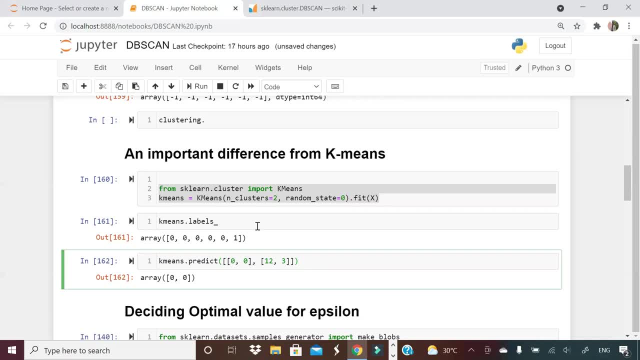 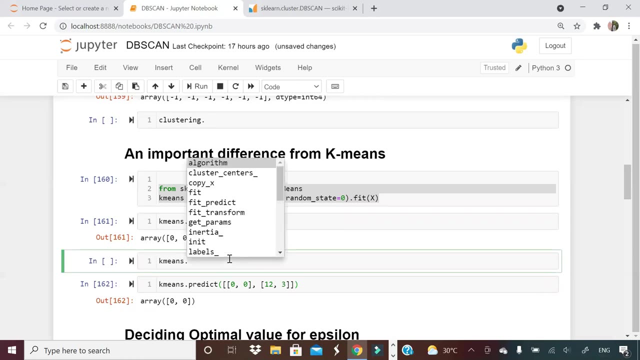 Now, one important thing to understand here is the way K-means clustering works is different from the way density based clustering works. guys, In K-means clustering your centroids are fixed Okay. So you can say here K-means, K-means dot. You can see the cluster centers, guys. 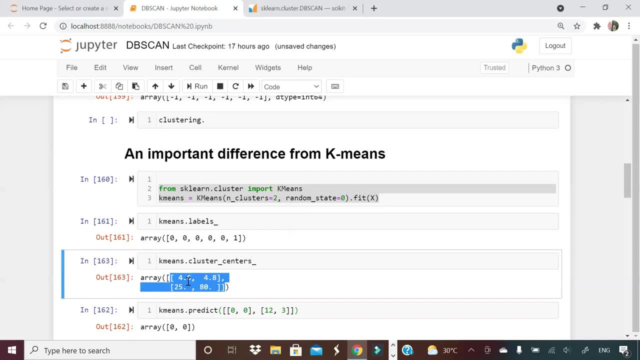 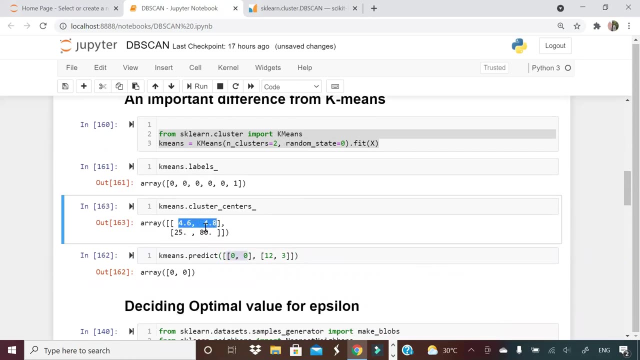 Okay, So these are your centers. Tomorrow a new data point comes right. It will just see these centers and see, okay, from which center these data points are closer. Now you can see here very easily that zero, zero is more close to this data point, or 2580.. Obviously. 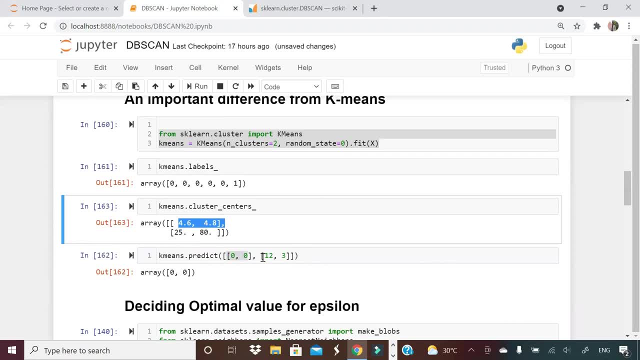 this data point right? That is where it is saying zeroth cluster, 12 and three. which data point it is closer? Obviously first one. that is where it says cluster number zero. If I make it something closer to 25 and 80, let me make it 24 and. 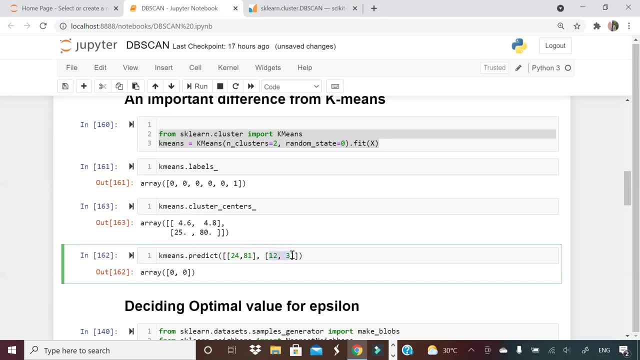 81. And here let me, let me make it a little closer to 25 and 80.. Okay, So 24 and 85. Now I expect these two data points to be assigned to second cluster. So this zero, zero should. 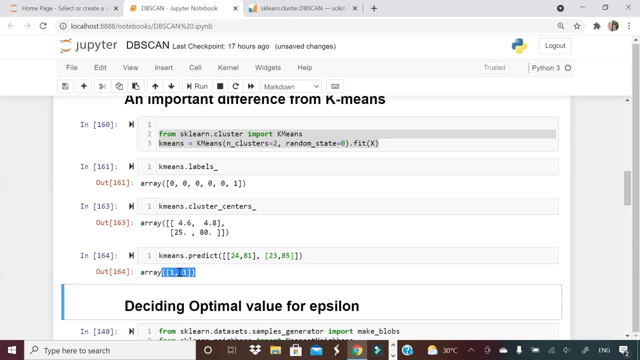 change to one one. Let's see It is changing to one one. The reason for that is: I want to make sure that our cluster centroids are fixed and you can predict on the new data point. but how density based clustering, or DBS, can work, says your cluster centroids are. 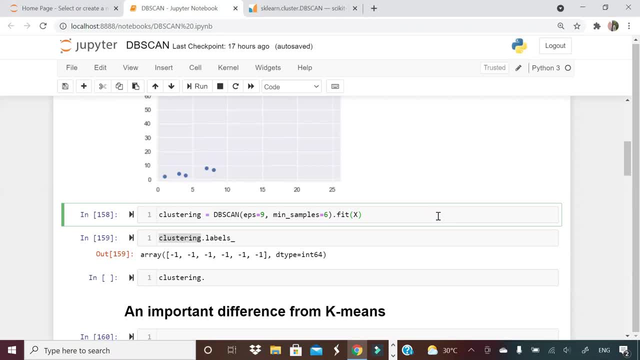 not fixed guys. Okay, It is working on a different way. It assumes that you will give it all the data point in one shot. It will see the densities and it will tell you: okay, this is one cluster, This is other cluster And you define what you define epsilon and you. 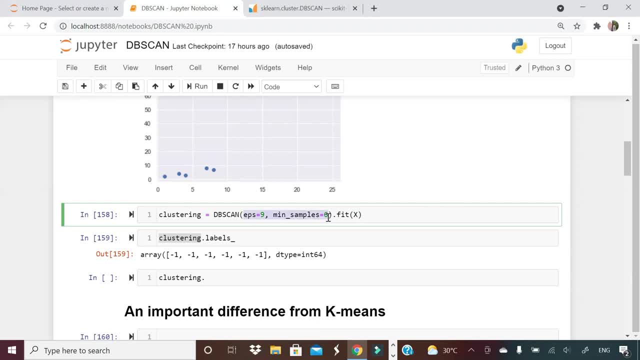 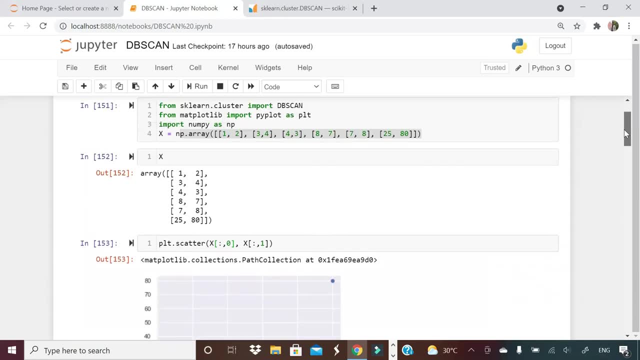 define minimum number of samples. Okay, Okay, So one important difference in DBS can clustering. You cannot predict on the new data set. Rather, if you want to create see in which cluster new data set falls, you need to rerun the. 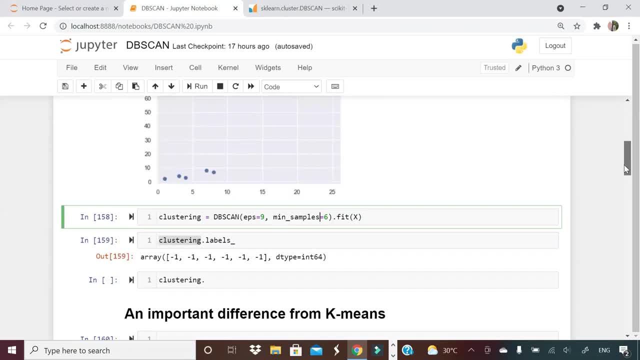 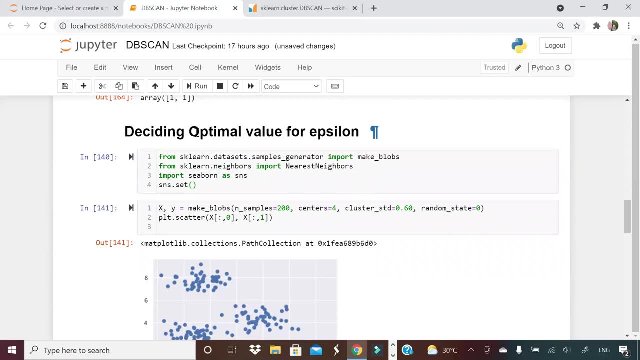 cluster one more time, Okay, But in K means you can predict on the new data point. So this section, which is part three of this video, I'm showing you deciding optimal value for epsilon. Okay, If you see, here I'm importing some, some libraries to generate some data. 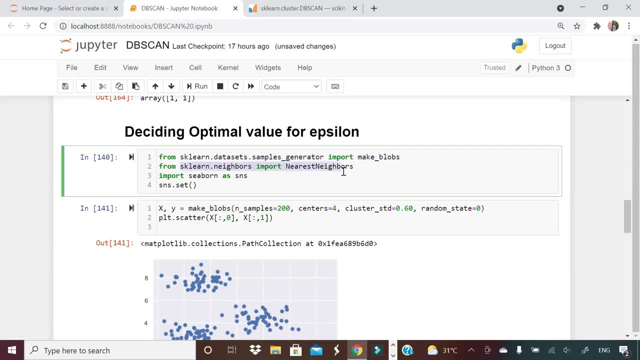 points and I'm importing from sklearn Something known as nearest neighbors. What is the use of nearest neighbor? I will tell you in a moment some seaborne to see some visualization. So what is the use of make blobs? is it will create some data points using SK. learn which. 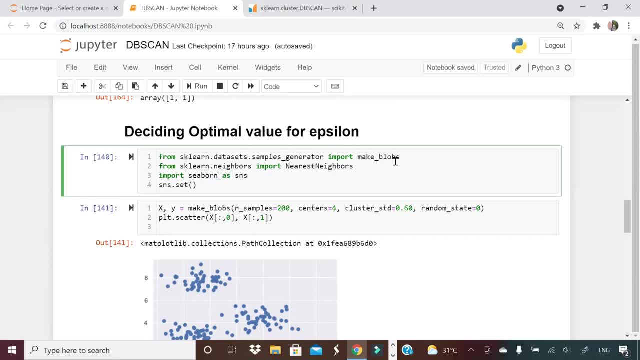 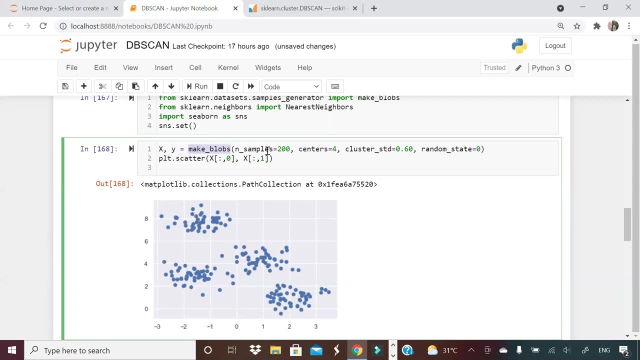 will have a, you know, cluster kind of arrangement. So did we run this and let me show you here If you see I'm generating X and Y by, by calling: make blocks function. How many points, Two points, how many centers, four, what is my cluster standard deviation? six point six. so what i'm doing, 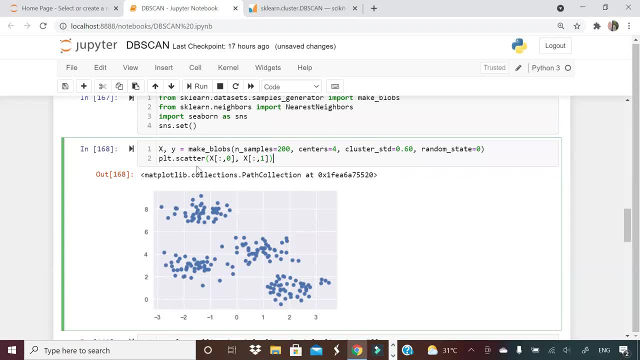 here, guys. you can think i'm just generating some data suitable for clustering. that's all i'm doing. okay, don't bother much about this. okay, just generating some data to suit for a clustering algorithm. you can take a data from a file also, not a problem. now i'm going to show you what does. 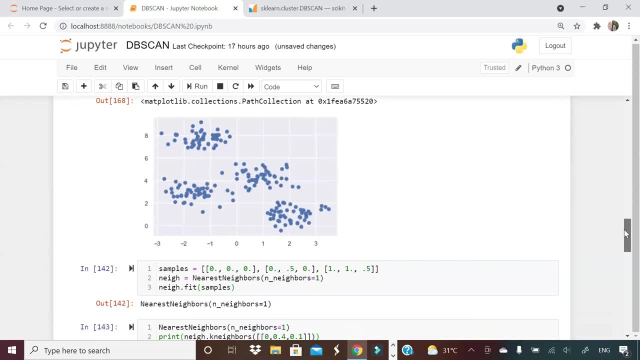 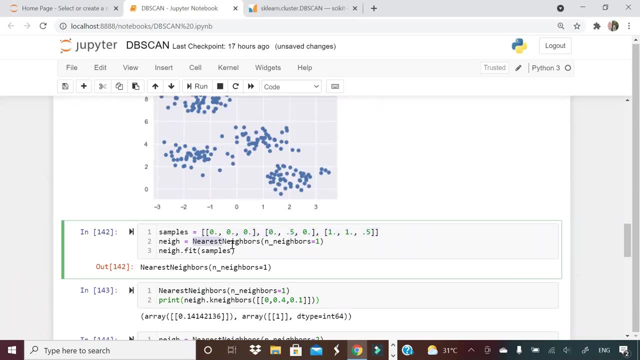 this nearest neighbor, do guys? okay, so come here. if you can see i have defined three data points here. okay, three data points here and i'm calling nearest neighbor here and i'm saying nearest neighbor is equal to one and fit on my samples. this is just a demo of what this module does, okay. 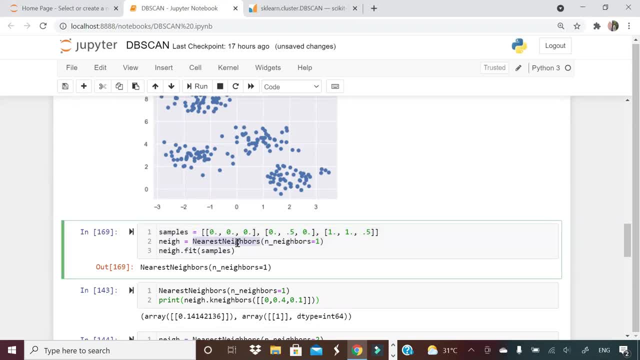 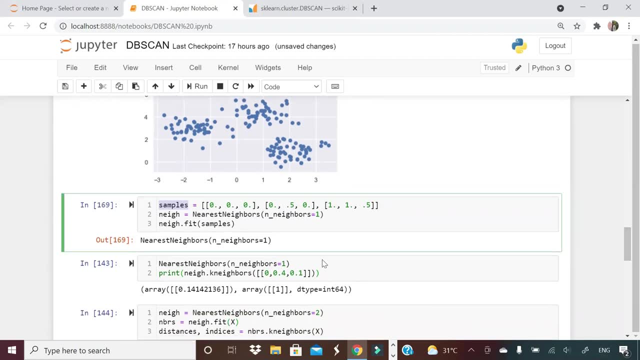 let me run this once. i fit this nearest neighbor on this samples data, then what i can do is i can give a data point as input, okay, okay. so if you can see here any igh is my model, i am saying dot k neighbors of this data. what is my? 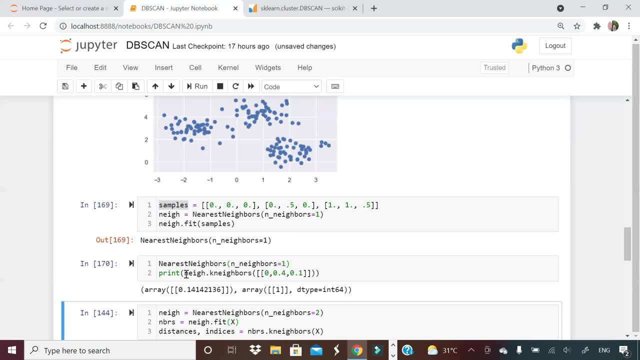 data: zero, zero point four, zero point one. let me run this, then you will understand. so zero, zero point four and zero point one is closer to which of these data points? guys tell me: zero, zero point four and zero point one is closer to which of these data point? second, second entry: right that. 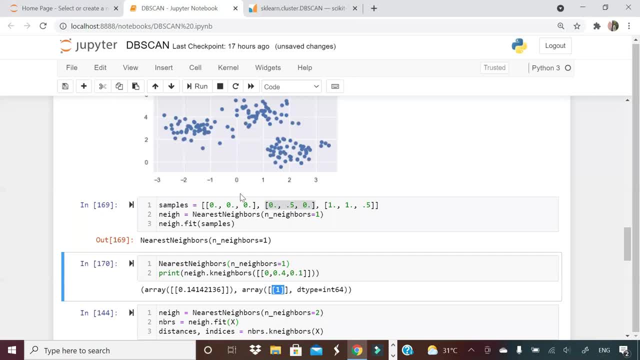 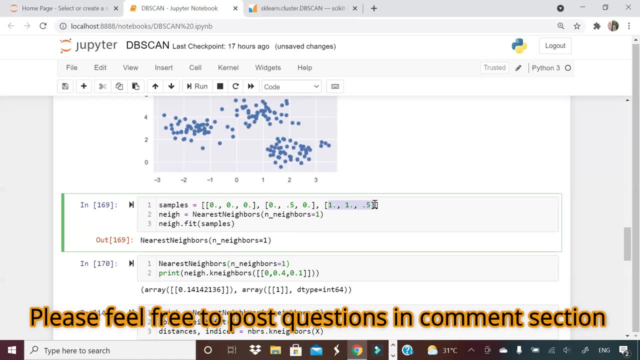 is what it says. array one one means you can start the zeroth index. this is zeroth thing. this is first thing and this is second thing. okay, so what nearest neighbor algorithm does is it will calculate the distance from all the data points and it will tell you- hey, you know what the data point you have supplied to. 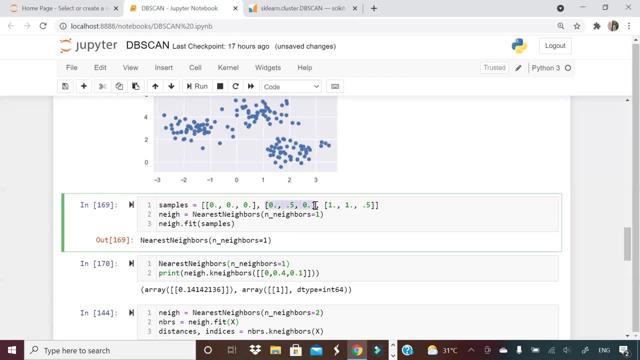 me, is closer to this one and the distance is zero point one four. okay, if i change this value, guys, let me try printing something which is closer to zeroth point. okay. so let me make it zero point one, second dimension. make it zero third dimension, keep it zero point. 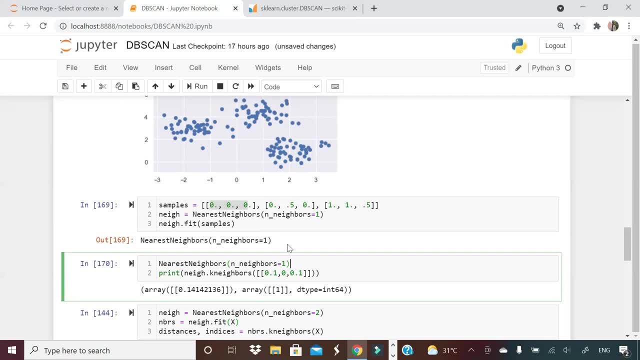 one. what i'm expecting is this: this observation should be closer to array zero, which means first, first entry in this samples okay, and distance also it will give. so, as you can see, array zero and distance also it is giving. so the crux of this is the job of nearest. 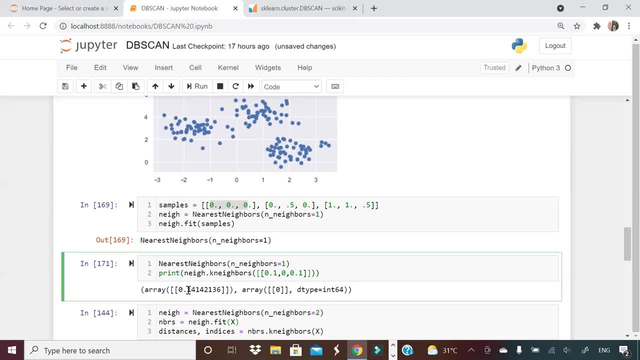 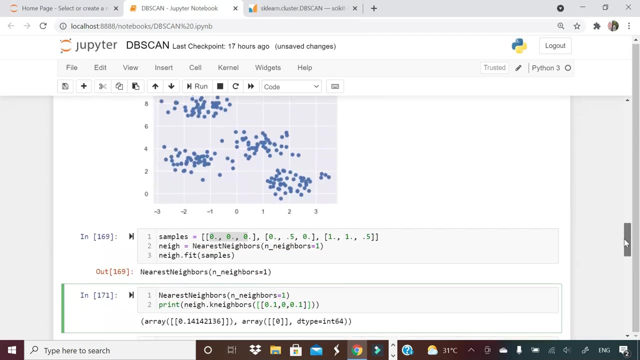 neighbor is to tell you in your population which data point is more close to which data point at and what is the distance between them. now what i am doing here, guys, i take all the data points from my above created data. okay, i am showing you how to indirectly derive the good value of epsilon. 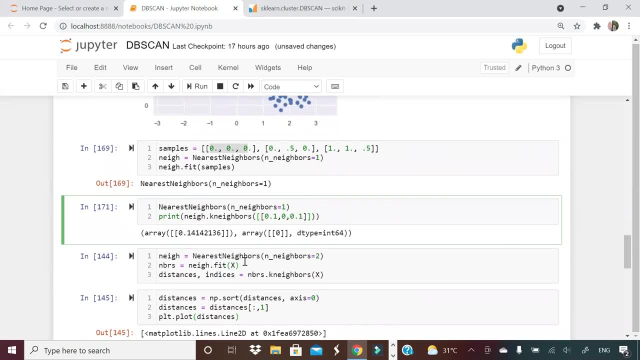 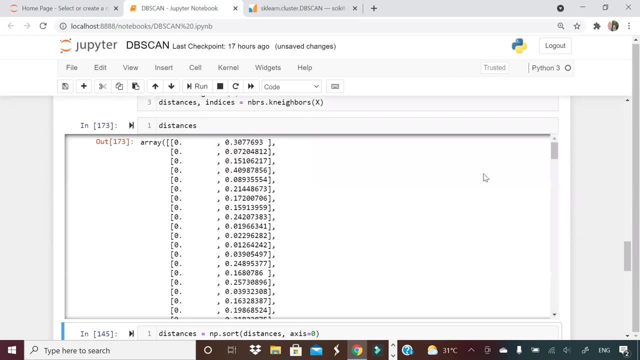 okay. so here i am fitting the same algorithm: nearest neighbor is equal to two, neighbors is equal to fit distance indices: neighbors dot neighbor. so if you see this distance, guys, let me run this, i will tell you what is this graph just a moment. so if you see this distance, right. 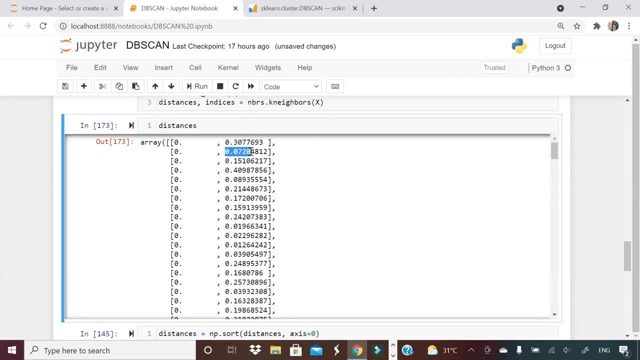 it tells you that this is the distance first one, this is the second one, this is the third one, this is the fourth one and, if you see the indices right, it tells you that between which two points it is calculating distance: point number zero and point number 62. that was the first entry in the 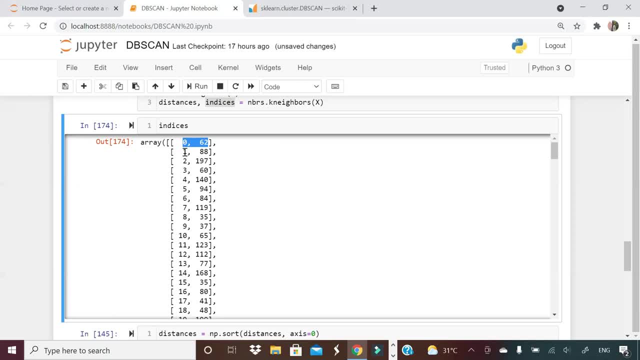 distance: uh, distance vector, uh, point number one and point number 88. the value that you saw just before. the second value was the distance between these two points. so what i am trying to find out here is in which distance range, in which distance range most of the distances are falling within that. 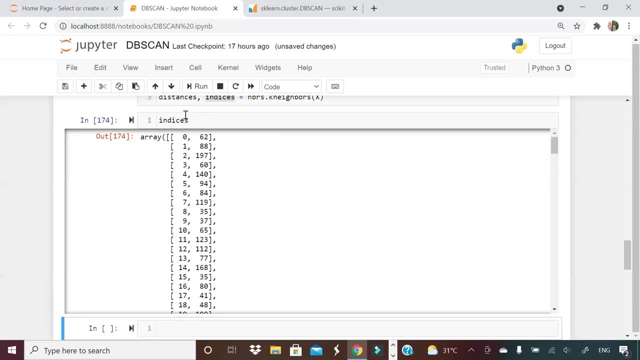 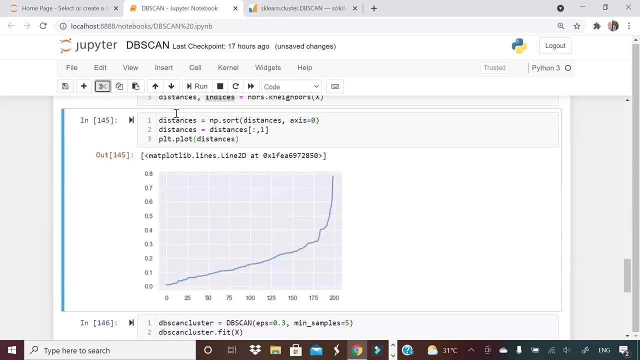 data. okay, so i take the distance, i shot it and i plot it. i take the distance, i shot it and i plot it. that is what i am doing here: np dot shot. take those distances, shot it and plot it. okay, so i take the distance, i shot it and i plot it and plot it and plot it. 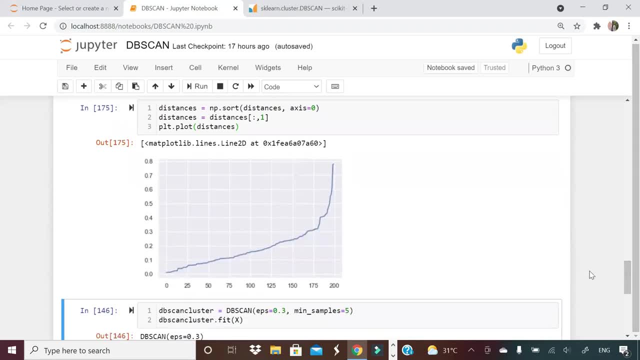 guys, what you are going to see here is, out of 200 data points, right out of 200 data points, the distance. the distance is mostly falling between, let's say, below 0.5 or 0.4, something like that. right so it is raising and after this, right it is. we cannot go for the value of distance. we cannot go at a very high level, right, if we go below this space, we cannot go for the value of. also, that is what i show you, right, if you plot it, that is how we solve this problem tree from here. so let's say, when this distance reaches point three, point three percent, the distance goes between 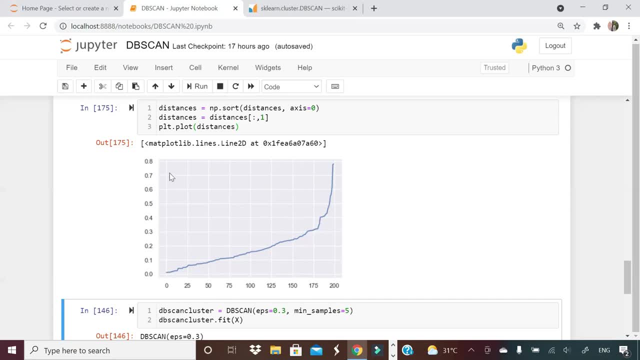 let's say, below zero point five or zero point four, something like that. right? so if we plot this point et away from the space, we can say, right here, based on the value you get here, theck, then we can use this space. yes, face value: very high level, then cluster will not make much sense. so we need to find out a point where there 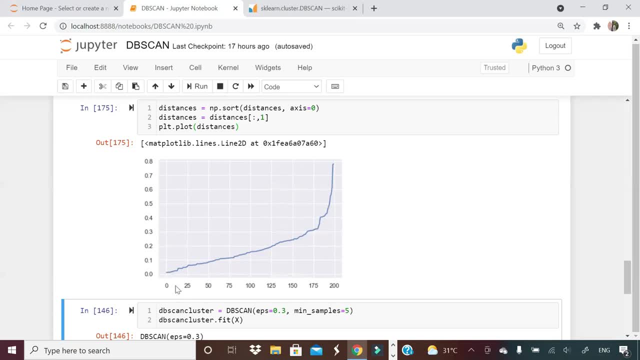 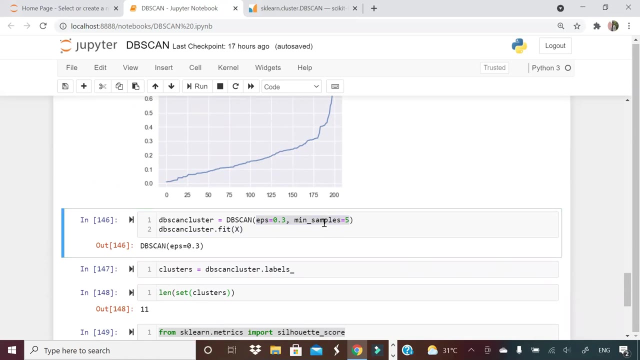 is a sharp increase or where there is a most percentage of points are covering. so here you can see 0.4, 0.5 are kind of candidates for that. so let me run db scan on this data with epsilon 0.3. first, epsilon 0.3 sample size. we are not optimizing minimum sample, so we will keep it. 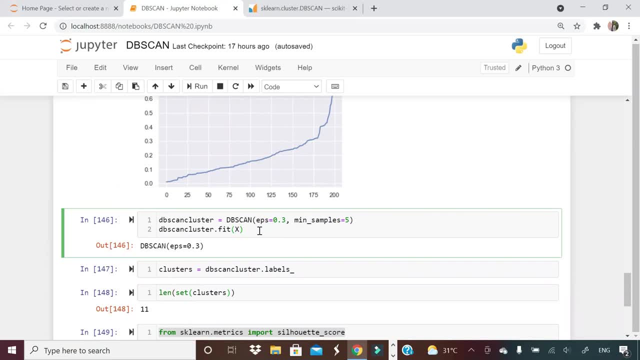 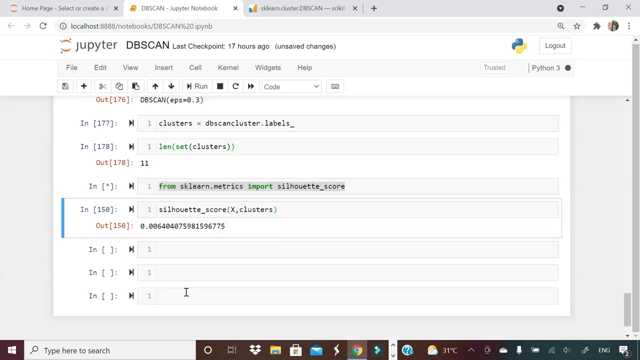 constant epsilon 0.3. let's see what happens. okay, we run. these are the cluster levels. now i have done a set and len that will tell me how many individual clusters are there. so 11 clusters. now. how do we verify goodness of our cluster using siloed score? what does the lot score say? 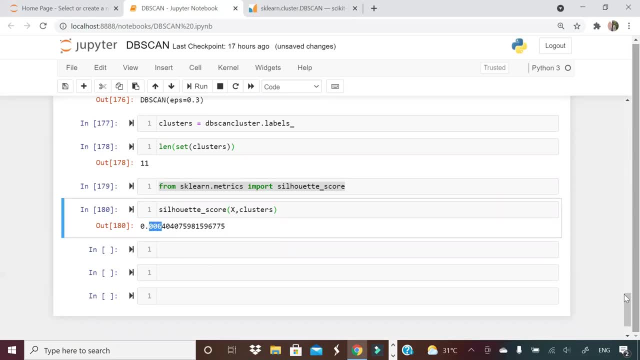 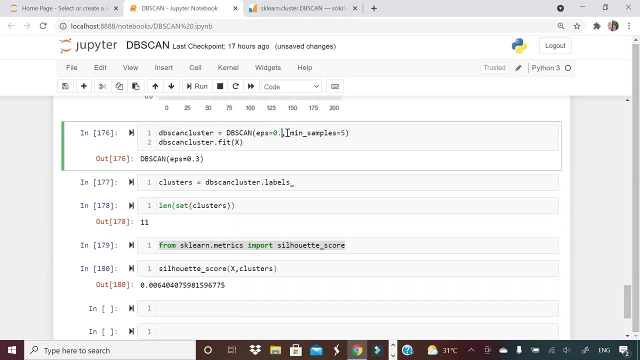 0.006, which means not a good cluster, okay, not a good clustering algorithm. i mean clustering model training. let us make epsilon 0.4 you. so what? what we are saying by making 0.4 guys? we are saying that consider something with the 0.4. 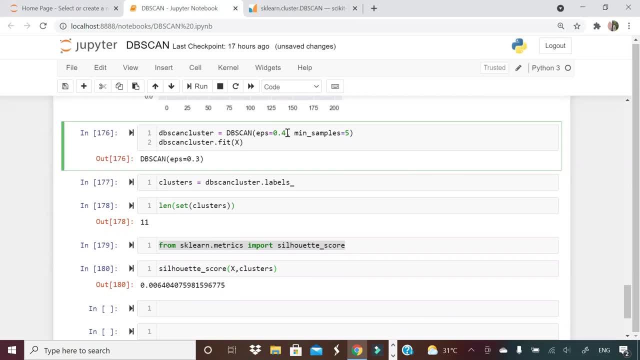 away also as the close. so number of clusters will increase or decrease. it will decrease, right. what is the slot now? 0.42, very good shift, right, very good shift. if i make it 0.5, epsilon, right, number of clusters will decrease further. here it is not decreasing. let's see what happens to. 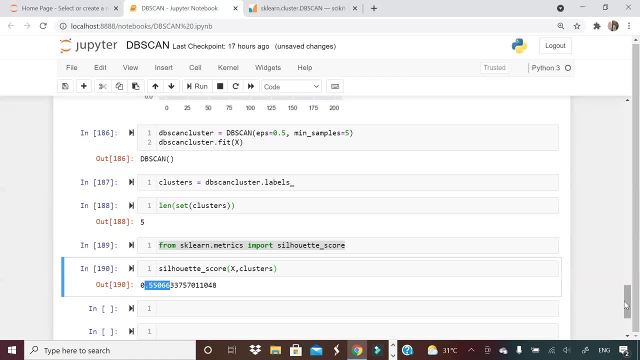 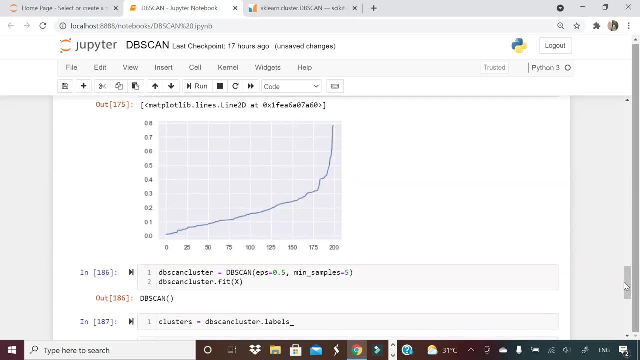 see lot 55, so it is increasing. so what i'm saying here is: more and more of your data points are in terms of closeness, right. in terms of closeness below 0.5 or 0.4, then that can be your one epsilon. 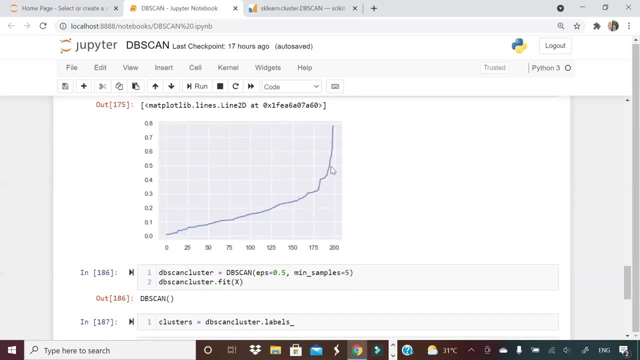 candidate. what you can do is you can run for different different things here. where there is a sharp, you know- shift, after covering some decent amount of percentage of your data right, that few of those epsilon you can take, run your clustering. check the clustering algorithm performance. 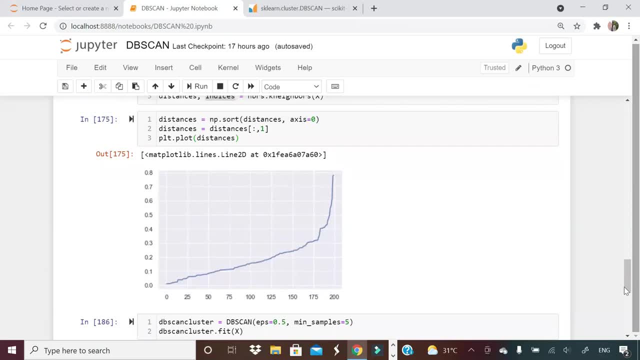 and then you can decide what is your epsilon. Okay, this exercise might be a little tricky If you have multiple dimensions and if you have more number of records in your data, but still very useful, guys. okay, Now I want to give you one simple assignment. Okay, what? 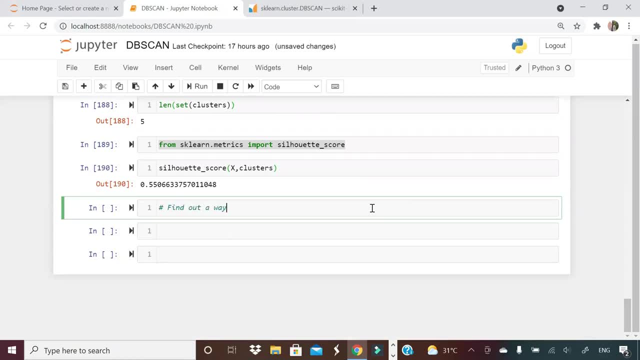 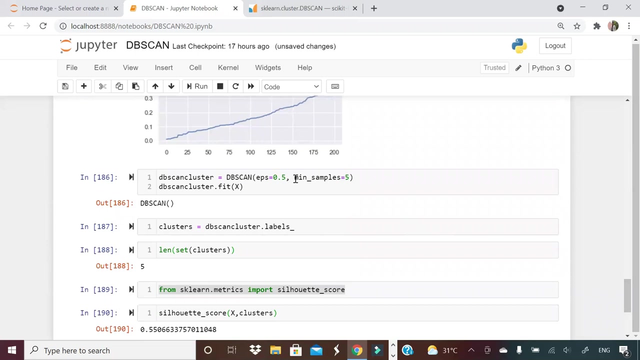 you have to do is you have to find out a way to get optimal maximum- sorry, minimum- number of sample, the other parameter. I mean to say, okay, minimum number of sample. So how do you do that? That? take that as an exercise and comment to me: how did you find you know?